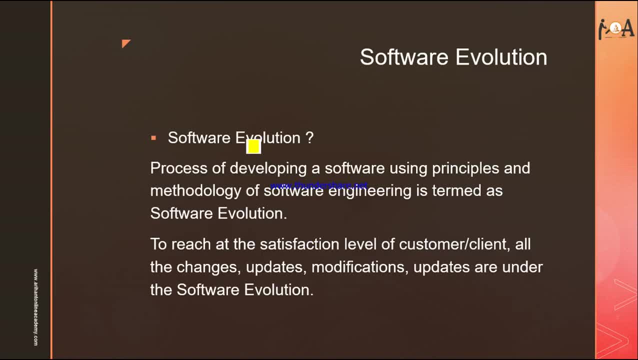 Software evolution. Basically, if we explore the term software evolution, then we can say that we have a software, Then according to the need of various users, various clients, Right. Or we can say that according to the use of customer, we have to modify the software, We have to update the software, Right. So by applying various processes, various methodologies, various principles. 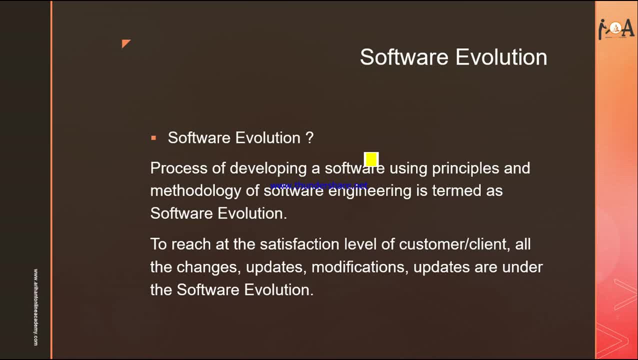 What we are doing? we are enhancing that software that is already existing. We are not getting it right again from very scratch or from very beginning every time, because it may find us very costly, Right? So what we are doing, we are making updates in a software, We are making enhancement in a software by applying various changes, various maintenance, so that the software can work as according to the need of customer or client. 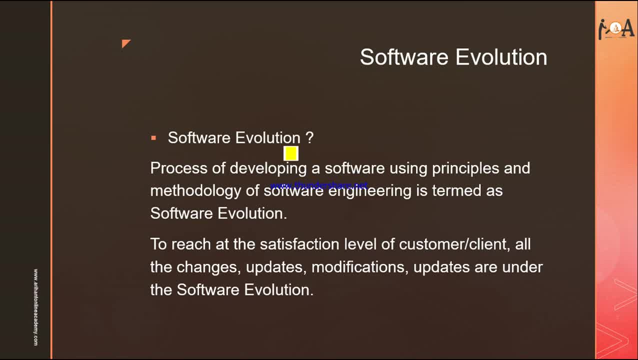 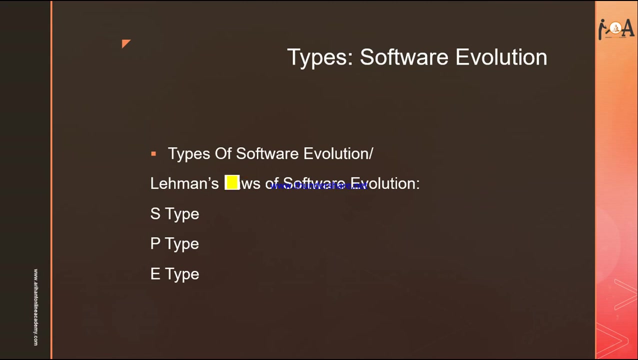 So this complete procedure is called as software evolution. Now let us see the definition. Why process of developing a software using principles and methodology of software engineering is termed as software evolution, To reach at the satisfaction level of customer or client. all the changes, updates, modifications or updates are under the software evolution. Now let us discuss the types of software evolution, or we can say that Lehman's laws of software evolution. Lehman basically puts three important laws, That is S type. 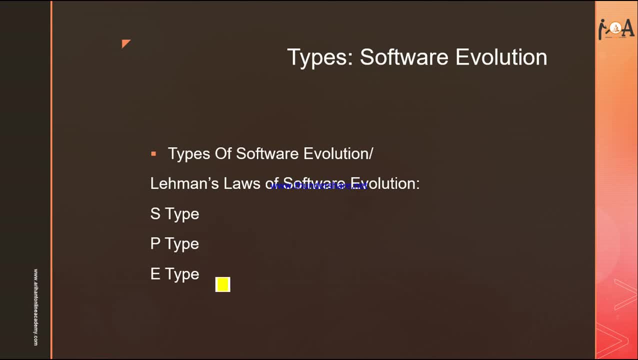 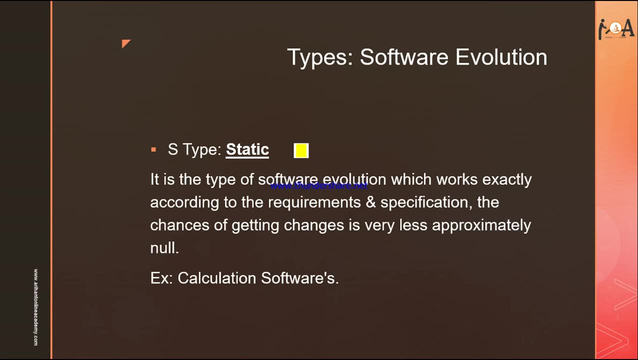 type, P type and E type. What are these three types of laws or the software evaluation types Let us discuss First. is S type, that is, you can say that static type. In this type of software evaluation it is work according to the specific needs or the requirements which 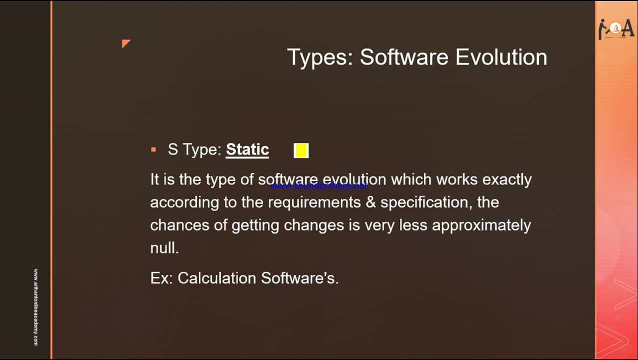 are. we have put at the initial level of our software development. So at the starting level of software development we are putting customers need that we have to make that software, we have to develop that software. So such kind of software is called as static software. 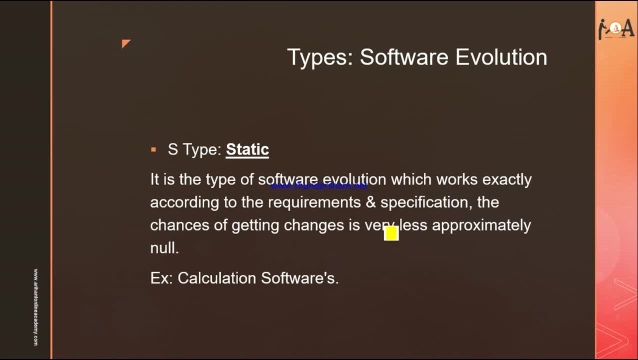 Means there isn't any further major changes at the last level. For example, a calculation software, or you can say that you have to make a calculator. So specifications are very specific, They are static right. So further there might not need any kind of changes. So this kind 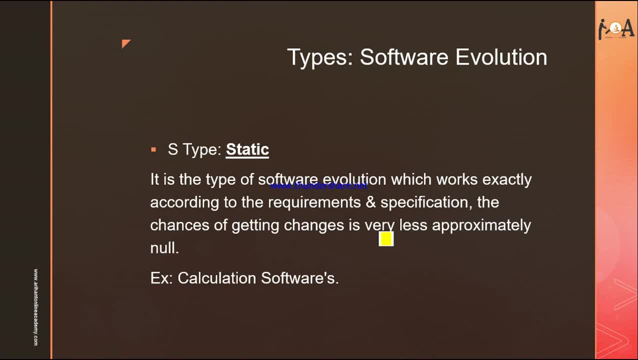 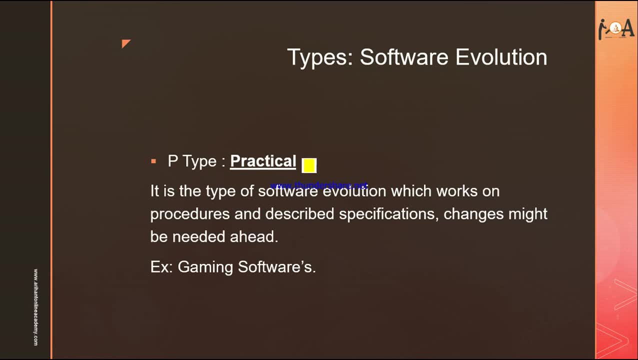 of changes. It is very. changes are very less or approximately null, or call as S type evolution or static type. The next is P type or you can say that of practical type. It is a type of software evaluation which works on procedures and described specification. changes might be needed ahead. 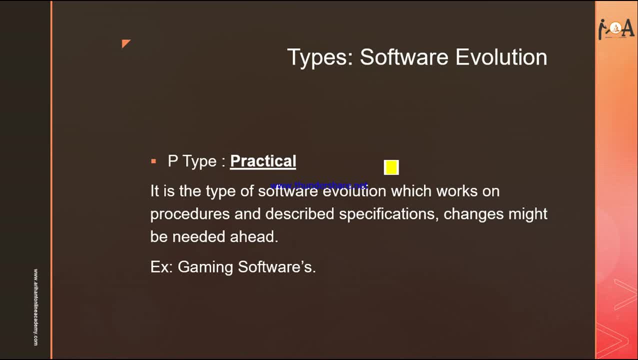 For example, you are developing a gaming software, Then in gaming software further, suppose at one level user complete, then after that you have to make the procedure that in next level you have to do, that you have to perform that, that after that you have to make some kind of locking software on unlock after completion of 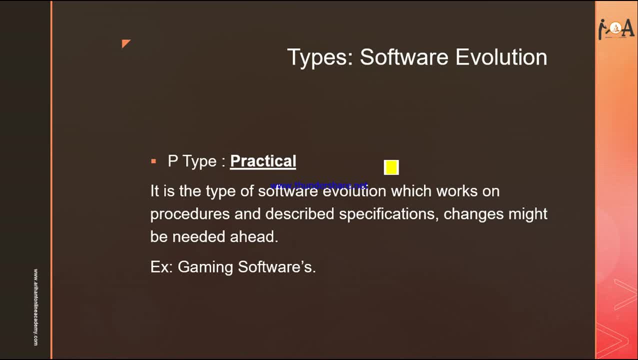 that level user only get throughout that level right. so basically, if you are applying procedures, means in next level it might get some changes. it might not need be, but changes might need not required in evolution, in solution of the next stage, right, but it might require in getting some. 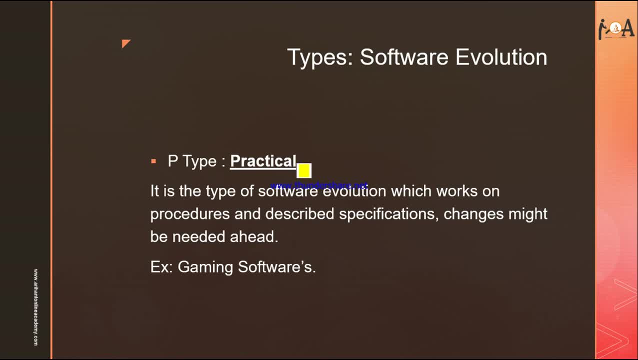 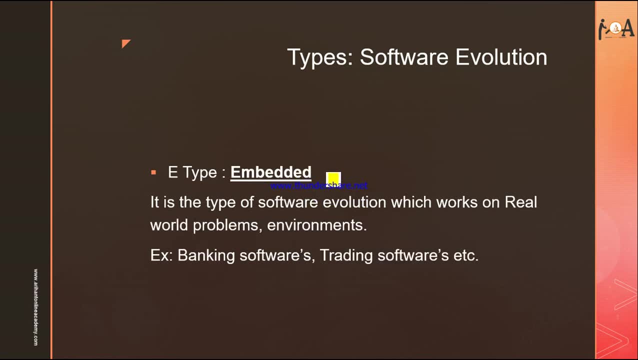 important update there. so it is a type of practical type, for example, gaming software. the next thing, very important is embedded type- e type. basically, in all this three types of lehman laws of software evolution, e type- that is, embedded type of software evolution- is very important it. 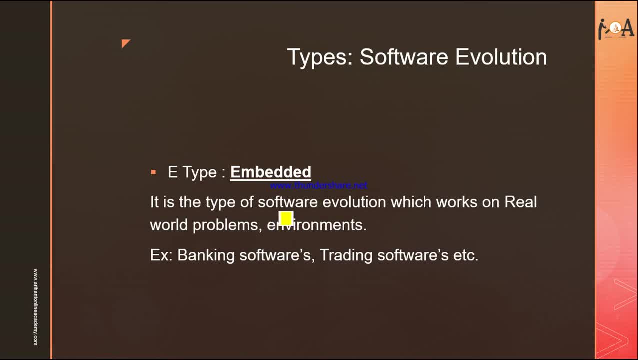 is a type of software evolution which works on real world problems, real environment problems, for example, banking softwares, trading softwares in real world environment, daily new kind of policy and policy wise. we can do some kind of practice like that. so it is a type of practical. 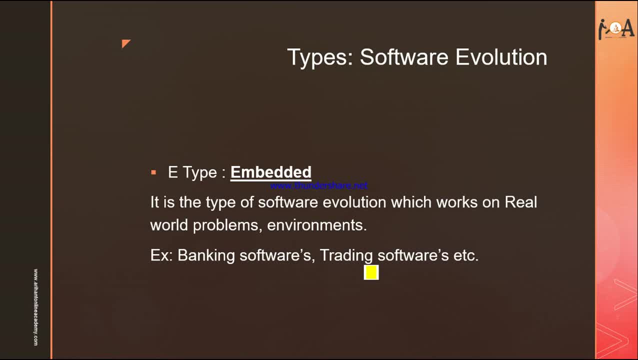 policies are coming, new taxes are coming, new kind of repo rates are coming. repo rates are updating, interest rates are updating. So you have to make software changes according to the environment, firstly in real world. So this kind of changes are called as embedded changes. 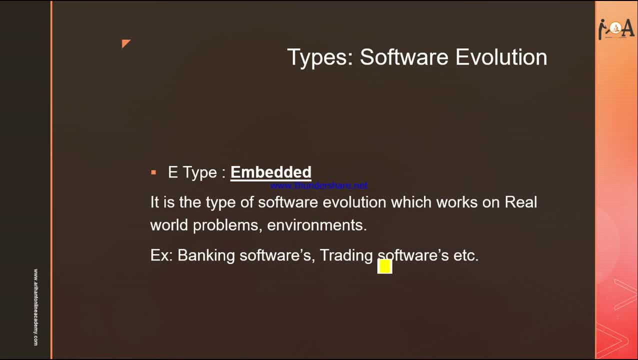 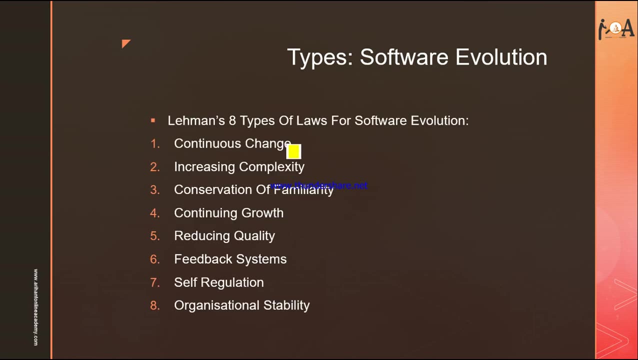 Trading software in which shares prices are getting down or upcoming in daily wise. So you are giving bonus to your customers, shareholders, So you have to maintain that in real world problem. So this kind of changes are called as embedded type. Now let's discuss the Lehmann's 8 types of laws for software evolution. 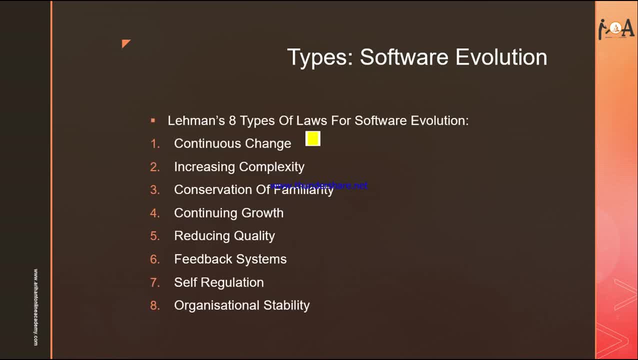 It is under E-type. It is under E-type right. That is embedded type. First is continuous change. What is continuous change? According to continuous change, we can say that it must continue adapt to real world change. If it will not adapt to the real world changes, then we can say that it will not work. according, 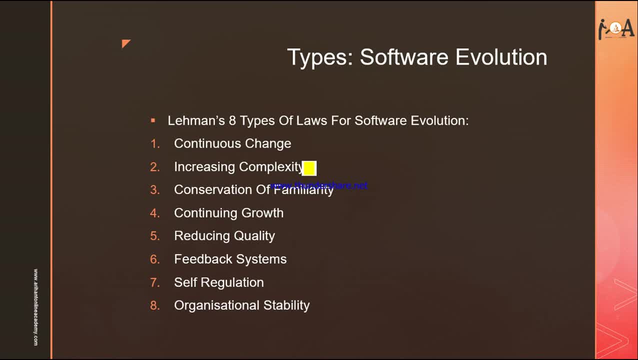 to the E-type right. The next is increasing complexity, Even though until and unless we will not maintain changes or E-type changes there, the software's complexity will get increased. So what we have to do, We have to maintain. We have to reduce the complexity by applying or evolving the increasing complexity by maintenance. 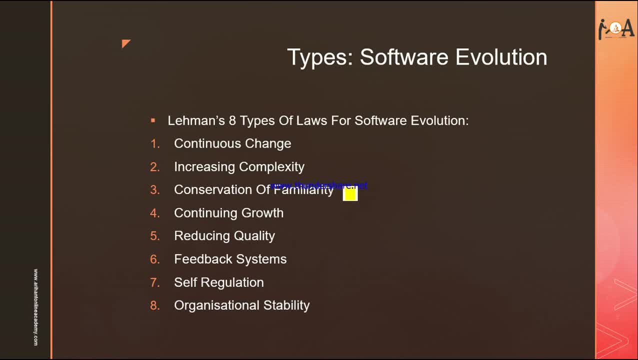 The next is conservation of familiarity. What is this? This term says that how the software is working. What about Why software is working? What is it working about? Means, what are the reasons on which software is working about? What are the software's parameters? right? 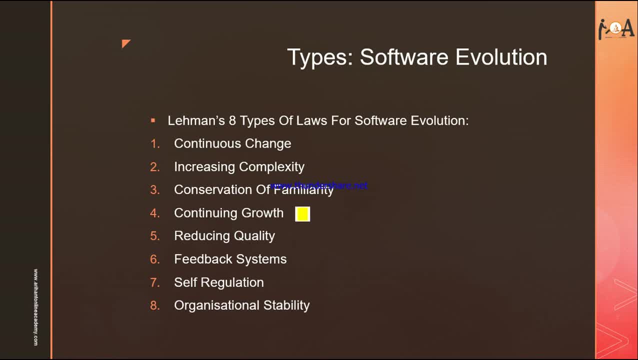 So all kind of this manners getting updated in conservation of familiarity. The next is continuing growth In order for an E-type system intended, or you can say that in a business type, growth according to the lifestyle changes of business. we have to make growth of software also. 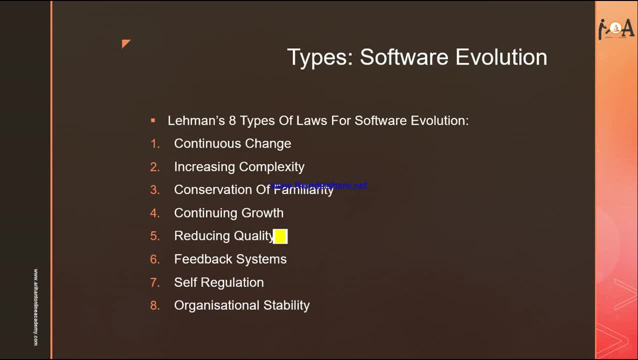 So this is E-type fourth principle of Lehmann's. The next is reducing quality. In reducing quality you can say that an E-type software system decline in software unless rigorously maintained or adapted to a changing environment. It is type of reducing quality. 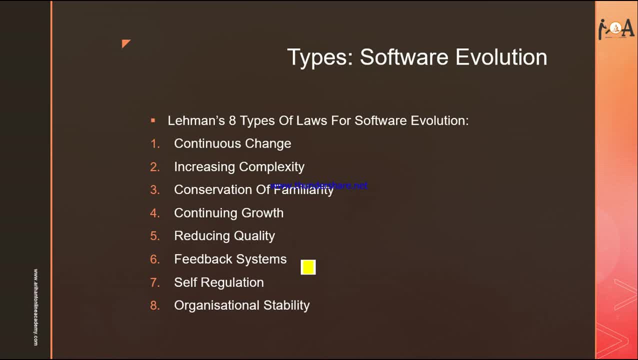 The next is feedback system. It is very important because the E-type software system constitute multi-loop, multi-level feedback system and must be treated as successfully modified, improved. The next is self-regulation. In self-regulation, E-type system evolution processes are self-regulating. 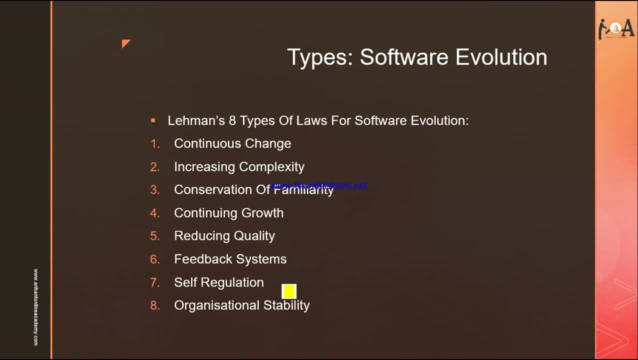 E-type system. evolution processes are self-regulating, With the distribution of product and processes measure close to normal. And the last, and very important, is organizational stability. It is the average of effective global activity rate in an evolving the lifestyle of the product. So these are the eight types of Lehmann's laws. 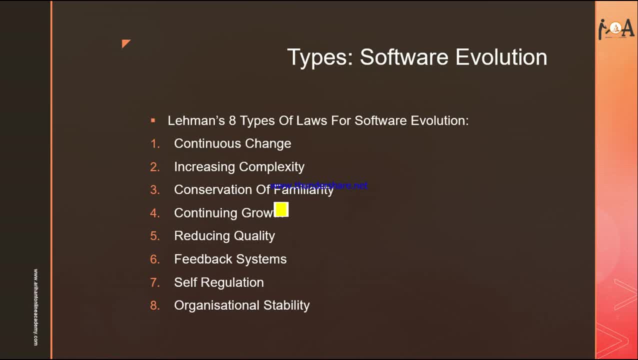 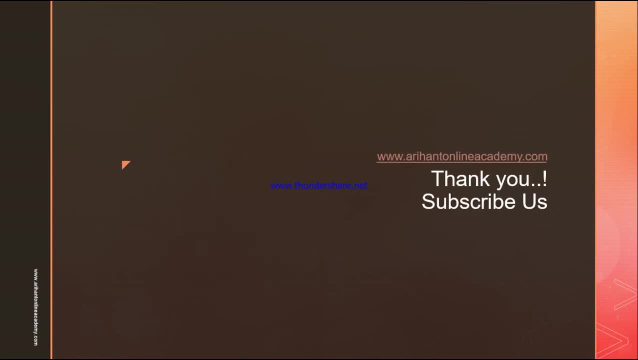 Basically, you need to just remember this- eight laws by their terminology. But for the explanation purpose also, I have explained all these terms Further. if you have any kind of suggestions or improvements or queries or any kind of doubts, you can comment us and we will try to improve or we will try to provide the solutions. 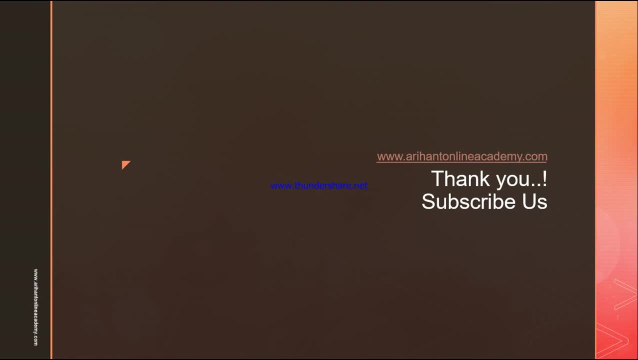 as early as possible. Thank you so much, guys. Have a nice day. Jai Hind, Jai Bharat.